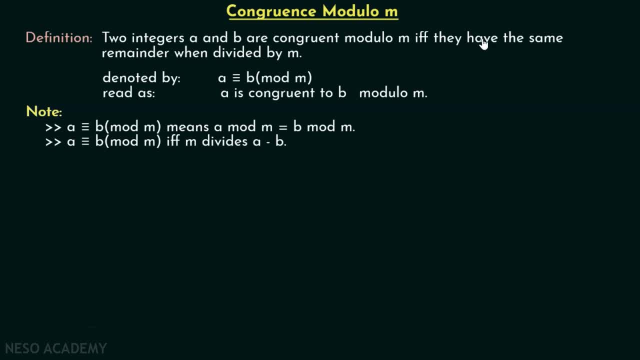 This is, according to the definition, right. They have the same remainder when divided by m. This means a mod m must be equal to b mod m. Apart from this, there is one more thing: a congruent to b modulo m if, and only if, m divides a minus b. 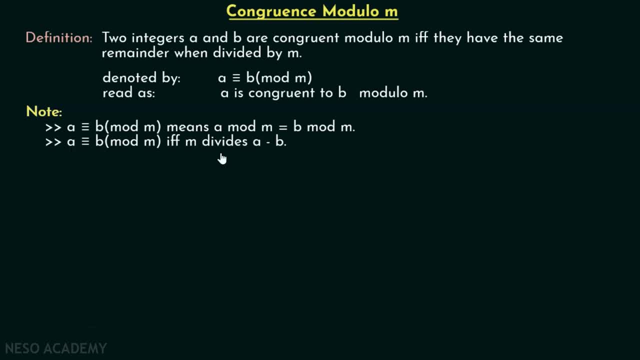 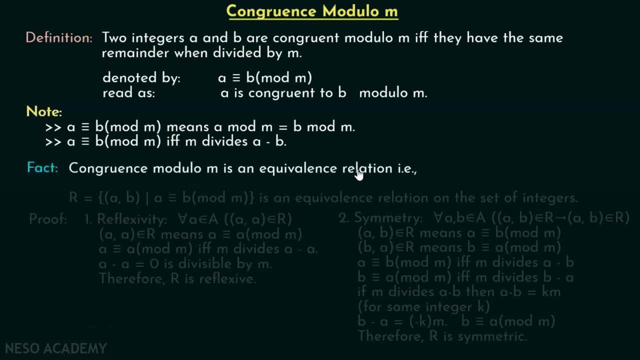 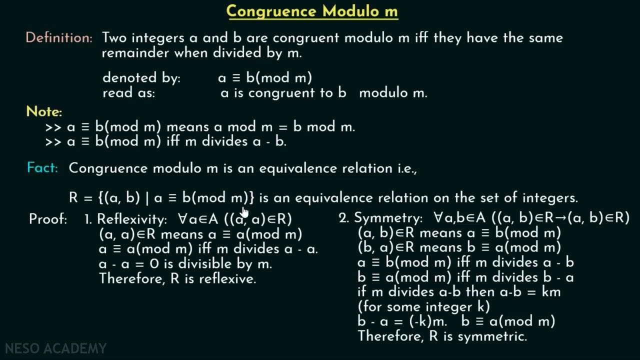 m divides a minus b. This is also true. Okay, Now here is one fact: Congruence modulo m is an equivalence relation, That is, r, which is equal to set of all ordered pairs, a, comma, b, such that a is congruent to b modulo m. 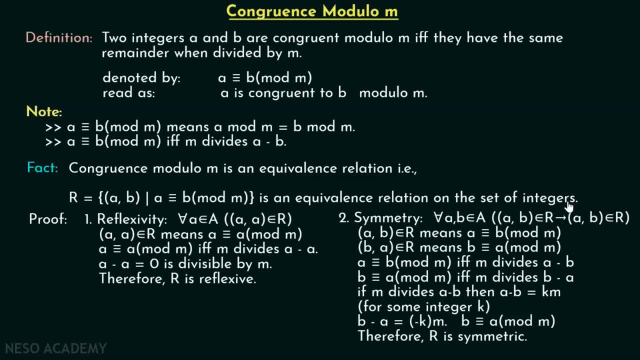 is an equivalence relation on the set of integers. This is the fact And we will try to prove this fact, Why this is so, Why this relation that is set of all ordered pairs, a, comma, b, such that a congruent to b modulo m. 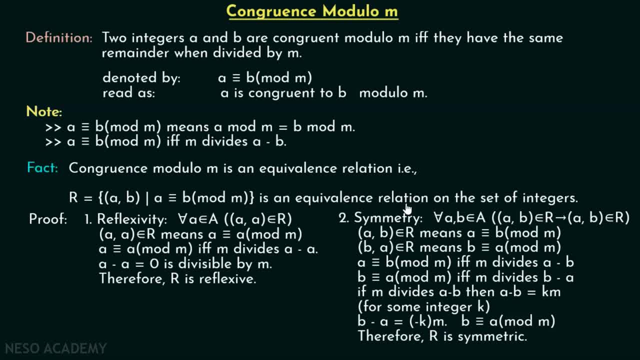 is an equivalence relation. For this, of course, we have to consider three properties of equivalence relation, That is, reflexivity, symmetry and transitivity. First we will apply the reflexive rule. That is, for all a belong to a. 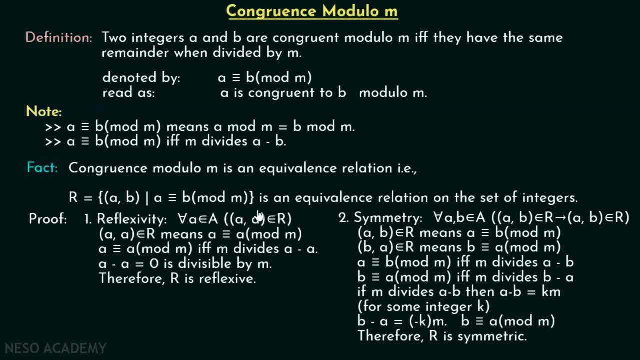 a comma a must belong to r, That is, this ordered pair must belong to this relation. a comma a belong to r means a is congruent to a modulo m. What do we mean by a congruent to a modulo m? a congruent to a modulo m means: 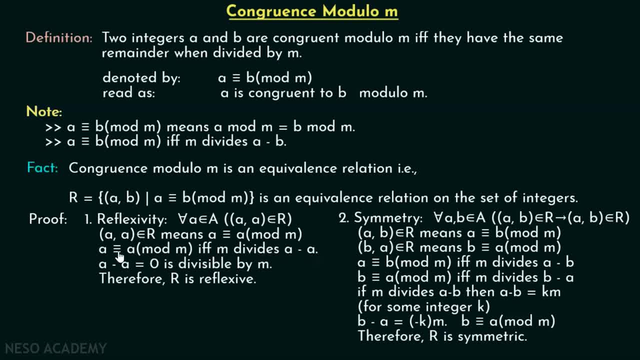 m divides a minus a Right a is congruent to a modulo m. if, and only if, m divides a minus a. What is a minus a? A minus a is zero, And zero is obviously divisible by m. It is divisible by any kind of integer. 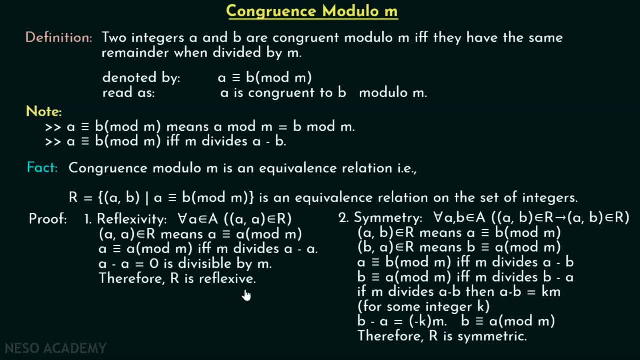 Therefore, r is reflexive, Isn't that? so Now let's see whether this relation is symmetric or not For all. a comma b belong to a. a comma b belong to r implies b comma a belong to r. What is the meaning of a comma b belong to r? 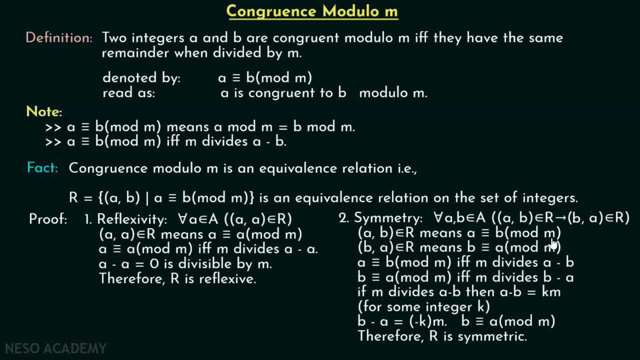 This means a is congruent to b modulo m. What is the meaning of b comma? a belongs to r Means b is congruent to a modulo m. If a is congruent to b modulo m, then b must be congruent to a modulo m. 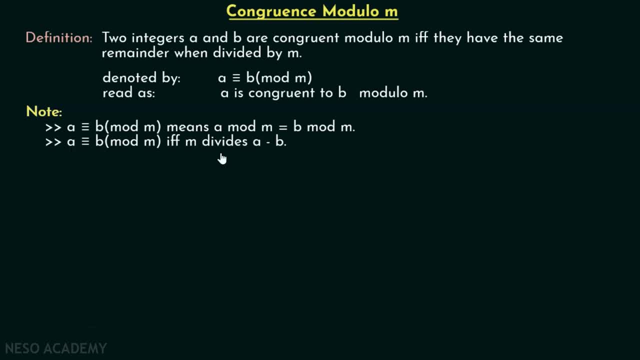 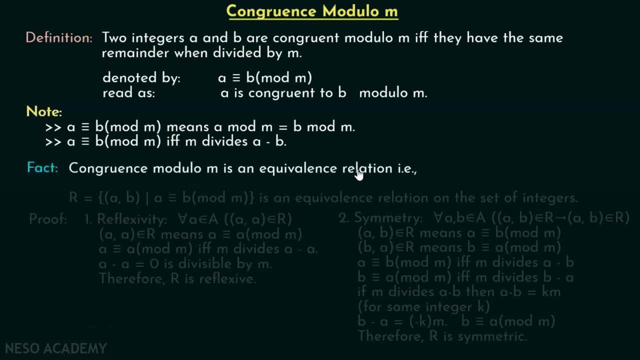 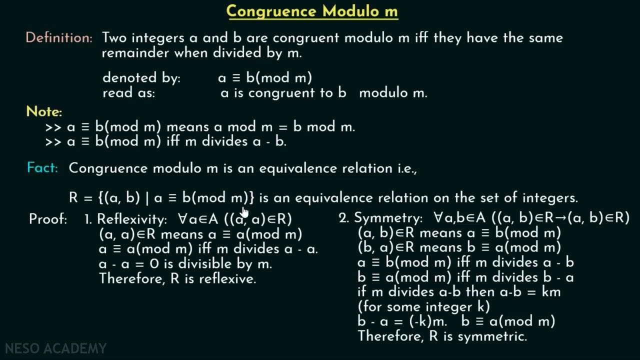 m divides a minus b. This is also true. Okay, Now here is one fact: Congruence modulo m is an equivalence relation, That is, r, which is equal to set of all ordered pairs, a, comma, b, such that a is congruent to b modulo m. 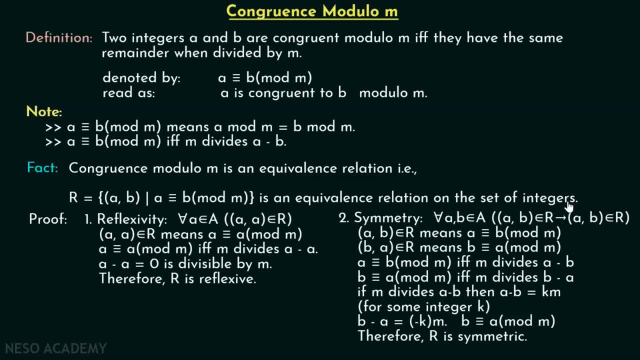 is an equivalence relation on the set of integers. This is the fact And we will try to prove this fact, Why this is so, Why this relation that is set of all ordered pairs, a, comma, b, such that a congruent to b modulo m. 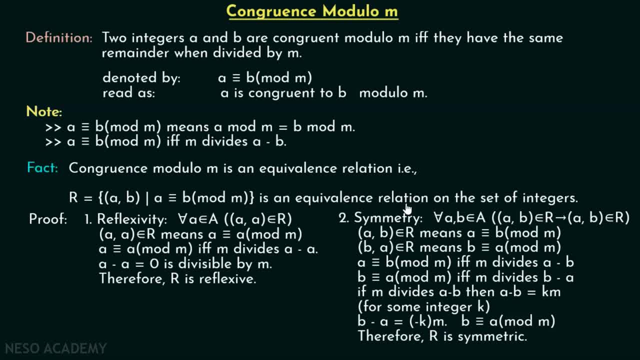 is an equivalence relation. For this, of course, we have to consider three properties of equivalence relation, That is, reflexivity, symmetry and transitivity. First we will apply the reflexive rule. That is, for all a belong to a. 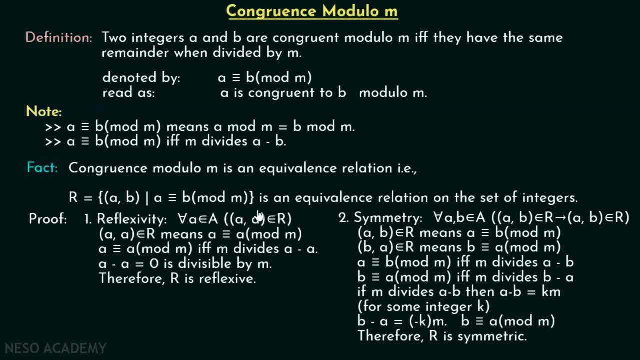 a comma a must belong to r, That is, this ordered pair must belong to this relation. a comma a belong to r means a is congruent to a modulo m. What do we mean by a congruent to a modulo m? a congruent to a modulo m means: 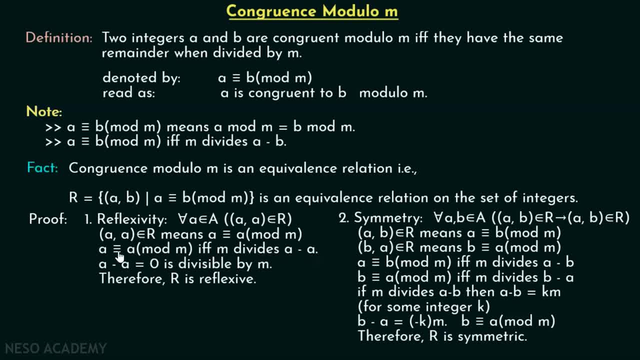 m divides a minus a Right a is congruent to a modulo m. if, and only if, m divides a minus a. What is a minus a? A minus a is zero, And zero is obviously divisible by m. It is divisible by any kind of integer. 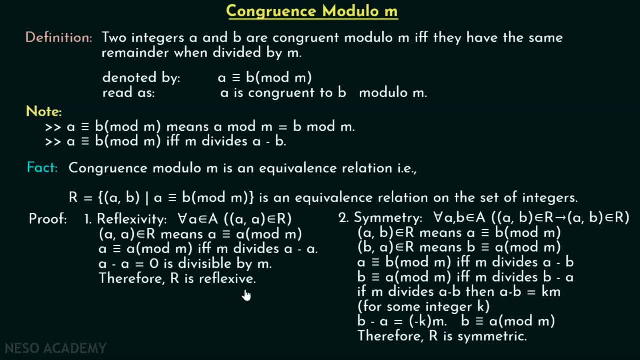 Therefore, r is reflexive, Isn't that? so Now let's see whether this relation is symmetric or not For all. a comma b belong to a. a comma b belong to r implies b comma a belong to r. What is the meaning of a comma b belong to r? 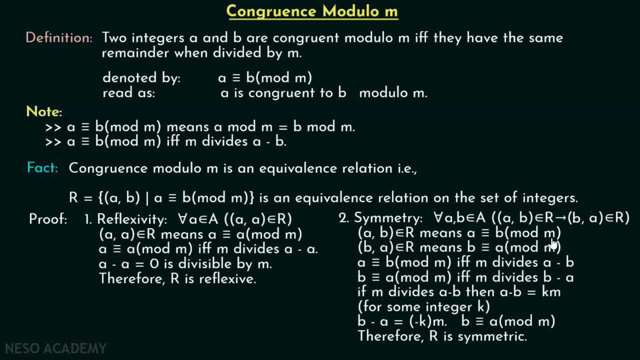 This means a is congruent to b modulo m. What is the meaning of b comma? a belongs to r Means b is congruent to a modulo m. If a is congruent to b modulo m, then b must be congruent to a modulo m. 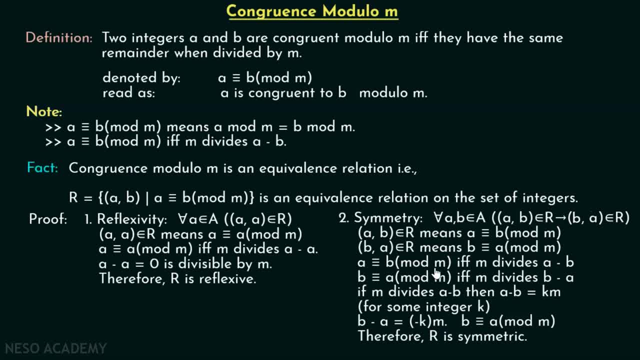 We know that, according to the definition, a is congruent to b modulo m if, and only if, m divides a minus b. And b is congruent to a modulo m if, and only if, m divides b minus a, If m divides a minus b. 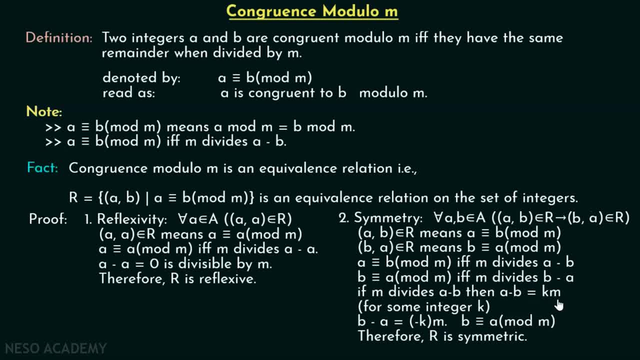 then a minus b must be equal to k into m. This is obviously true, because if a minus b is divided by m, then it will leave some integer. k Right k is some integer. In other words, we can say that a minus b is equal to k into m. 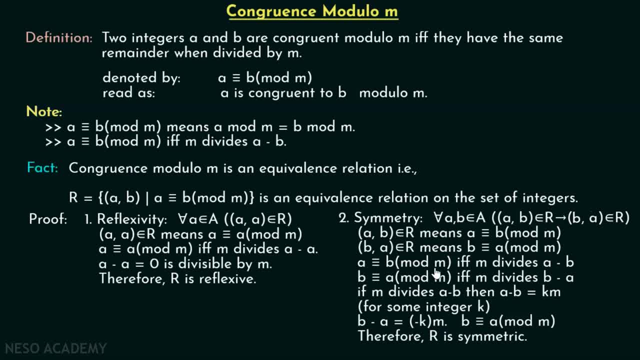 We know that, according to the definition, a is congruent to b modulo m if, and only if, m divides a minus b. And b is congruent to a modulo m if, and only if, m divides b minus a, If m divides a minus b. 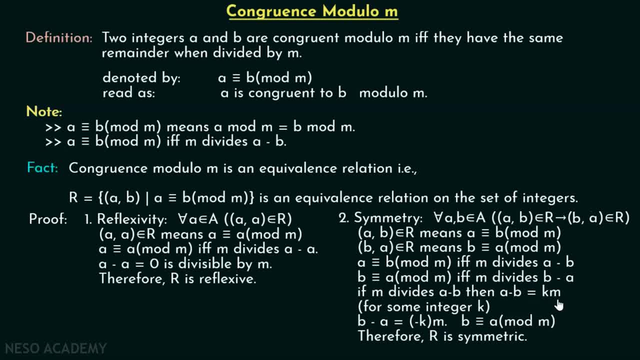 then a minus b must be equal to k into m. This is obviously true, because if a minus b is divided by m, then it will leave some integer. k Right k is some integer. In other words, we can say that a minus b is equal to k into m. 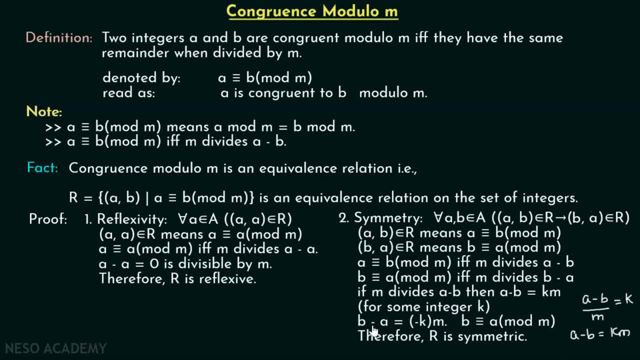 Right. For some integer k And b minus a is nothing but minus k into m. We can write in this form: Therefore: b is congruent to a mod m, Because minus k is also an integer Right. b minus a is also divisible by m. 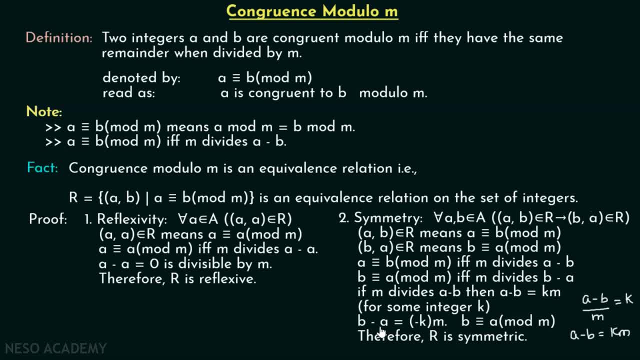 If a minus b is divisible by m, then b minus a is also divisible by m. Therefore, b is congruent to a mod m. And finally, this means that r is symmetric, Isn't that so? Let's see whether this relation 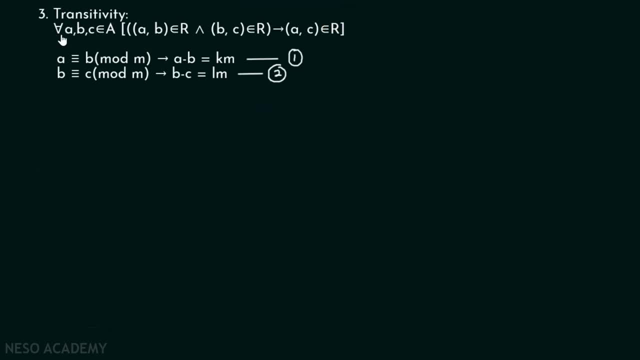 is transitive or not. According to transitivity, for all, a, b, c belong to a, a comma b belong to r and b comma c belong to r implies a comma c belong to r. Right Now we know that a comma b belong to r means. 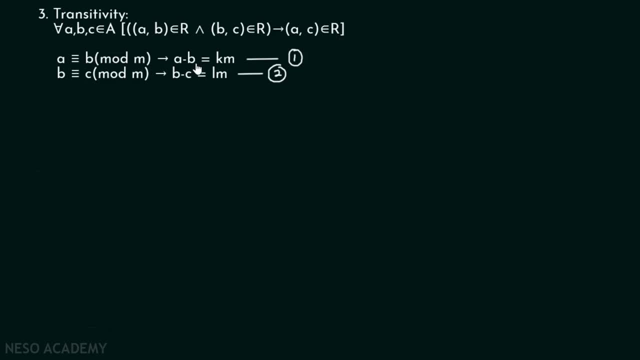 a is congruent to b mod m, Which implies a minus b equal to k into m. Right, That means a minus b is divisible by m. b congruent to c mod m means b minus c equal to l into m. for some integer l. 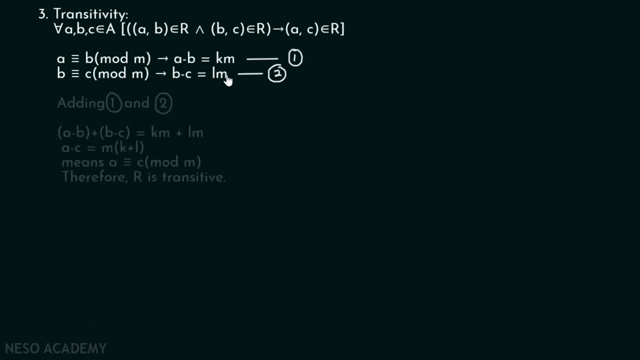 Let us suppose that this is 1 and this is 2.. Okay, Adding 1 and 2 gives a minus b plus b minus c, which is equal to k into m plus l into m. Right, We can take m common from both sides. 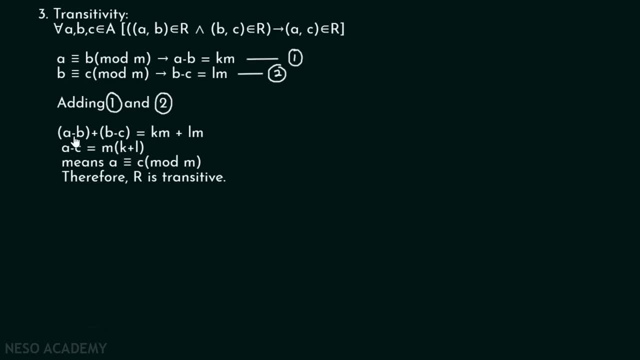 This will give us m into k plus l, and this is a minus b plus b minus c, which is equal to a minus c. So a minus c is nothing but m into k plus l. k plus l is also an integer. therefore a minus c is also divisible by m. 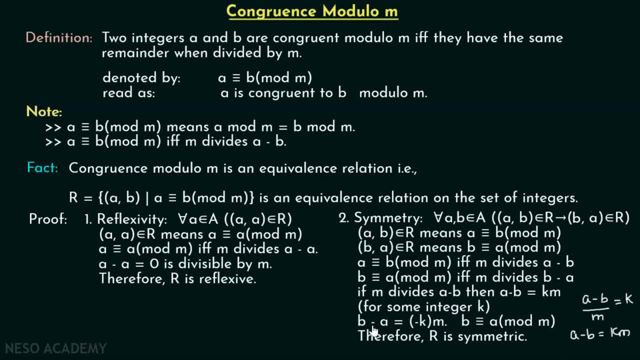 Right. For some integer k And b minus a is nothing but minus k into m. We can write in this form: Therefore: b is congruent to a mod m, Because minus k is also an integer Right. b minus a is also divisible by m. 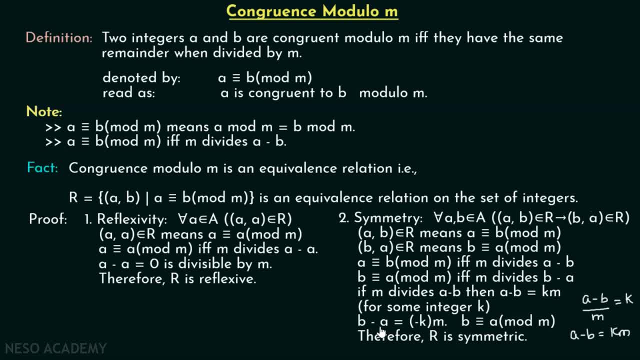 If a minus b is divisible by m, then b minus a is also divisible by m. Therefore, b is congruent to a mod m. And finally, this means that r is symmetric, Isn't that so? Let's see whether this relation 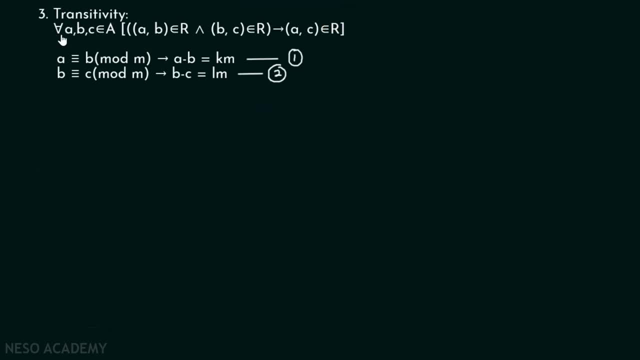 is transitive or not. According to transitivity, for all, a, b, c belong to a, a comma b belong to r and b comma c belong to r implies a comma c belong to r. Right Now we know that a comma b belong to r means. 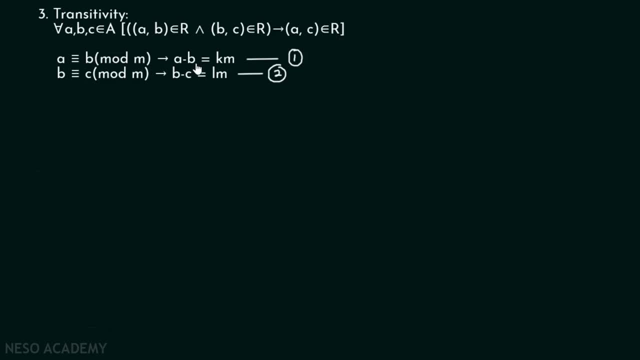 a is congruent to b mod m, Which implies a minus b equal to k into m. Right, That means a minus b is divisible by m. b congruent to c mod m means b minus c equal to l into m. for some integer l. 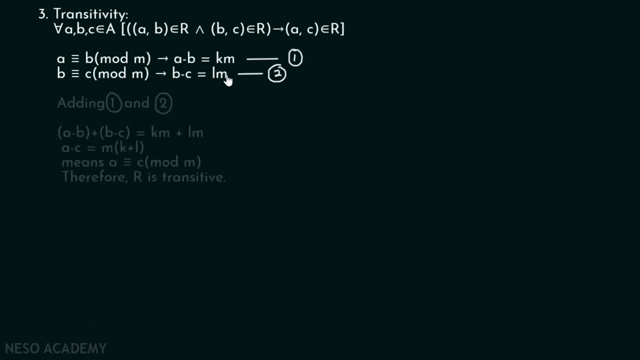 Let us suppose that this is 1 and this is 2.. Okay, Adding 1 and 2 gives a minus b plus b minus c, which is equal to k into m plus l into m. Right, We can take m common from both sides. 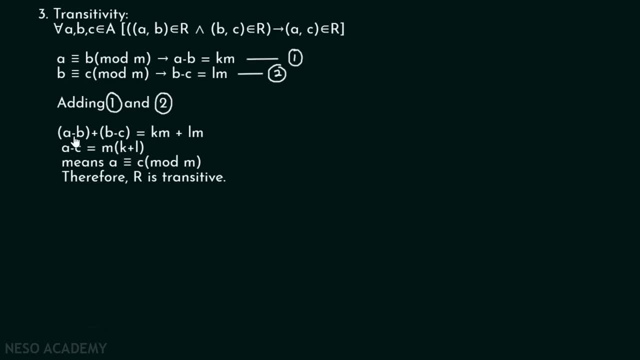 This will give us m into k plus l, and this is a minus b plus b minus c, which is equal to a minus c. So a minus c is nothing but m into k plus l. k plus l is also an integer. Therefore a minus c is also divisible by m. 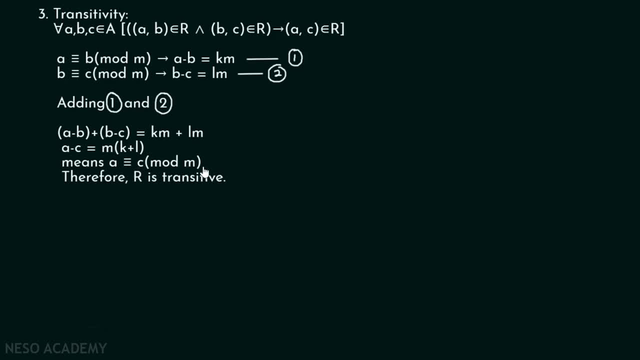 which means that a is congruent to c mod m. Therefore, r is transitive, Isn't that? so It is clear that r, which is nothing but set of all ordered pairs, a, comma, b, such that a congruent to b mod m, is an equivalence relation. 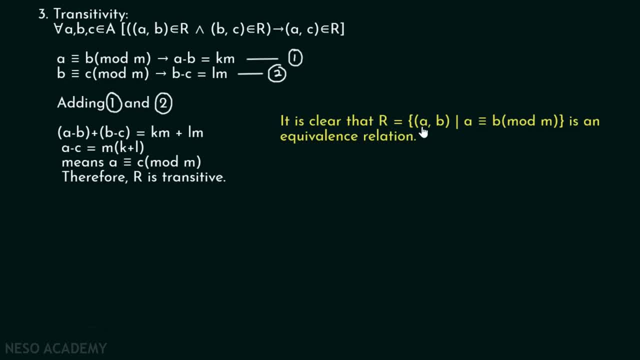 Right, That is it. r is an equivalence relation That is set of all ordered pairs a, comma, b, such that a congruent to b mod m is nothing but an equivalence relation. If this is an equivalence relation, we can also find the equivalence classes. 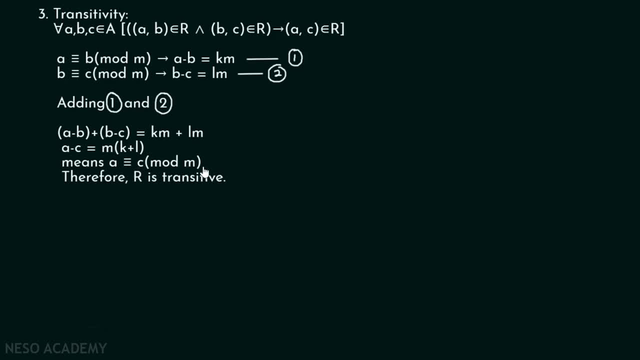 which means that a is congruent to c mod m. therefore r is transitive, Isn't that? so It is clear that r, which is nothing but set of all ordered pairs, a, comma, b, such that a congruent to b, mod m, is an equivalence relation. 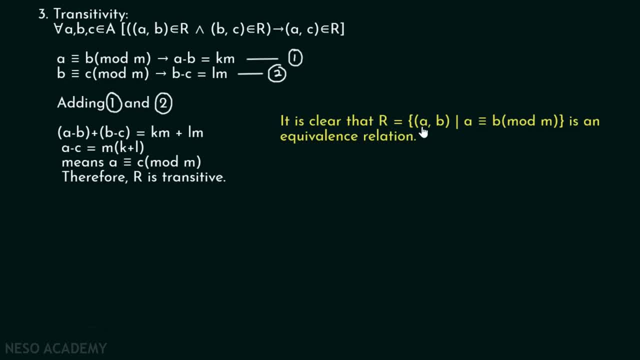 Right, That is it. r is an equivalence relation That is set of all ordered pairs a, comma, b, such that a congruent to b mod m is nothing but an equivalence relation. If this is an equivalence relation, we can also find the equivalence classes. 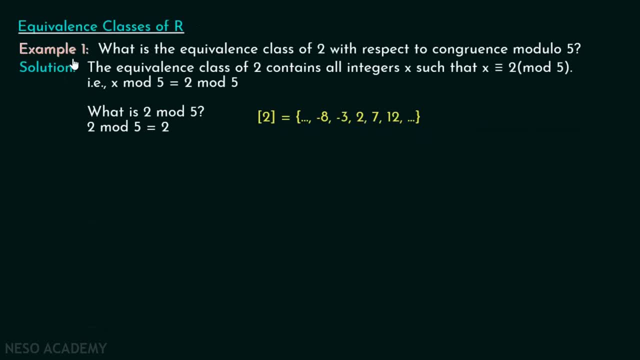 of this relation. Let's find out the equivalence classes of r. Let's consider one example. What is the equivalence class of two with respect to congruence modulo five? We want to find the equivalence class of two with respect to congruence modulo five. 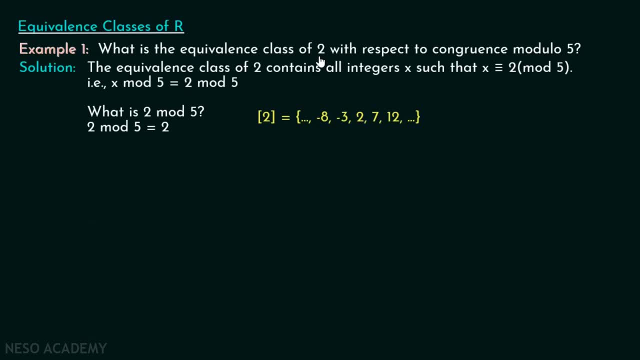 This is quite simple. We want to find the equivalence class of two, which means that we are interested in finding all the integers x such that x is congruent to two mod five. That is what we are interested in. This means x mod five must be equal to two mod five. 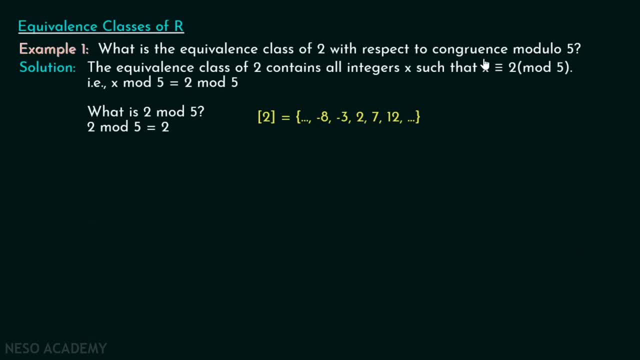 Question is asking us to find the equivalence class of two with respect to congruence modulo five. This means we are interested in finding all those integers x such that x is congruent to two mod five. This means x mod five must be equal to two mod five. 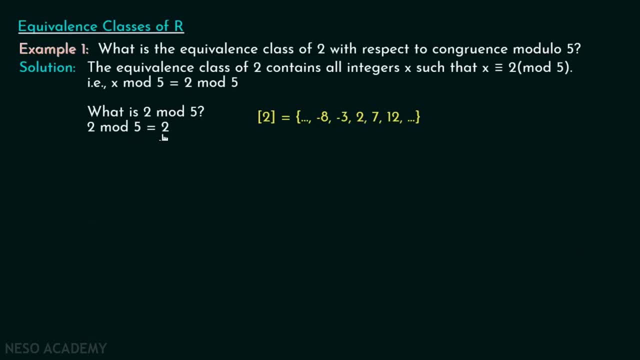 What is two mod five? Two mod five is nothing but two. Two, when divided by five, will leave the remainder two. We are interested in finding all those integers which will leave the same remainder. This will form the equivalence class of two. We know that two is related to two. 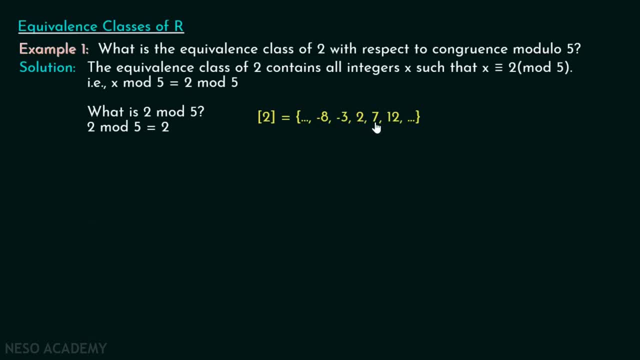 Therefore, two must be there in this equivalence class. Apart from this, seven must also be there in this equivalence class, because seven mod five is also two. Similarly, twelve mod five is also two. Also, minus three mod five is two and minus eight mod five is also two. 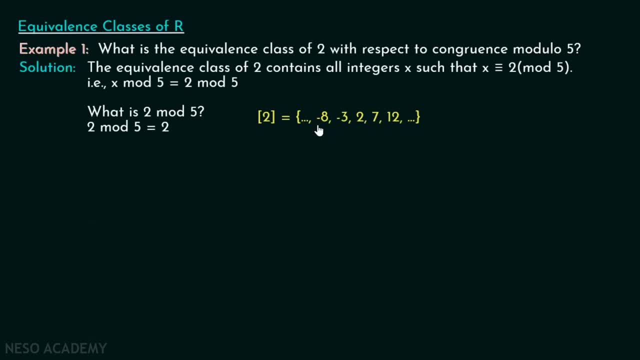 You can see that this is an infinite list, Right? And obviously this is an equivalence class of this element two. Let's see example two. What is the equivalence class of four with respect to congruence modulo five? We are interested in finding the equivalence class. 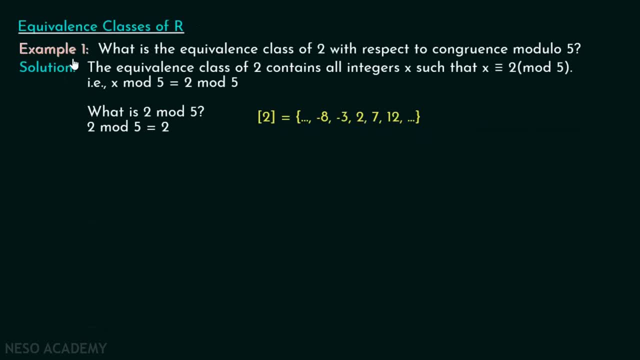 of this relation. Let's find out the equivalence classes of r. Let's consider one example. What is the equivalence class of two with respect to congruence modulo five? We want to find the equivalence class of two with respect to congruence modulo five. 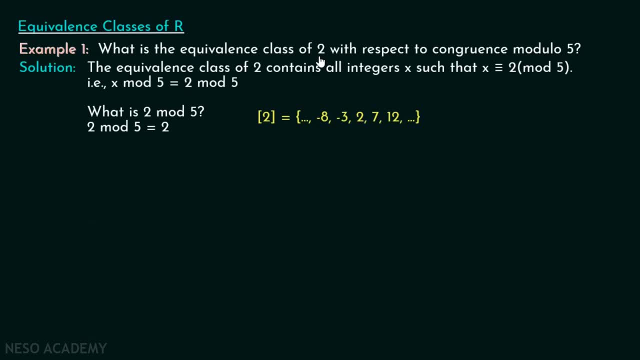 This is quite simple. We want to find the equivalence class of two, which means that we are interested in finding all the integers x such that x is congruent to two mod five. That is what we are interested in. This means x mod five must be equal to two mod five. 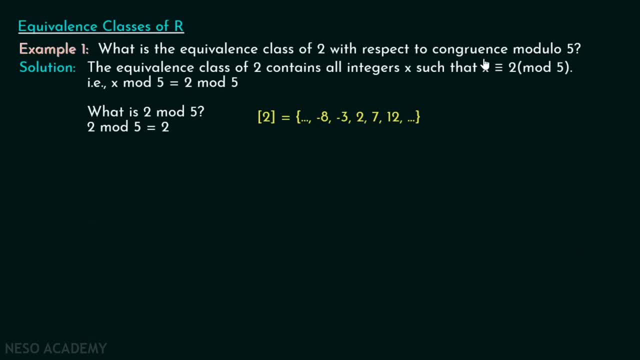 Question is asking us to find the equivalence class of two with respect to congruence modulo five. This means we are interested in finding all those integers x such that x is congruent to two mod five. This means x mod five must be equal to two mod five. 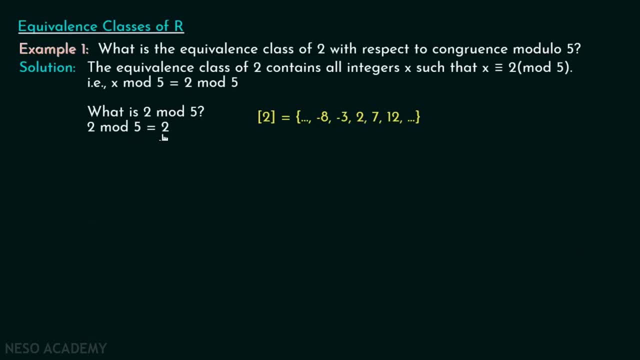 What is two mod five? Two mod five is nothing but two. Two, when divided by five, will leave the remainder two. We are interested in finding all those integers which will leave the same remainder. This will form the equivalence class of two. We know that two is related to two. 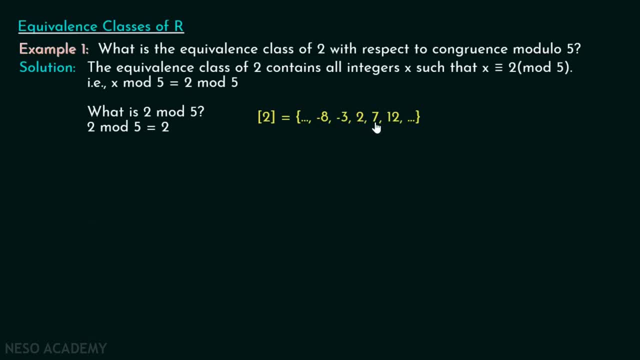 Therefore, two must be there in this equivalence class. Apart from this, seven must also be there in this equivalence class, because seven mod five is also two. Similarly, twelve mod five is also two. Also, minus three mod five is two and minus eight mod five is also two. 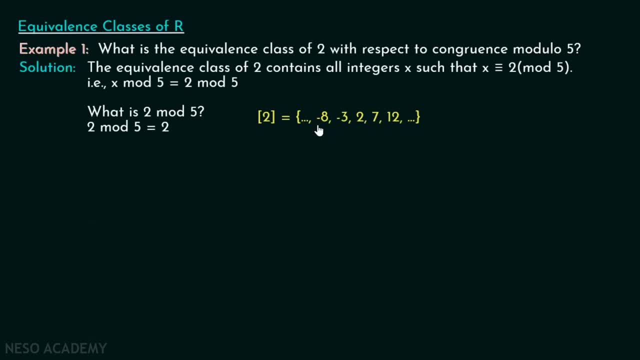 You can see that this is an infinite list, Right? And obviously this is an equivalence class of this element two. Let's see example two. What is the equivalence class of four with respect to congruence modulo five? We are interested in finding the equivalence class. 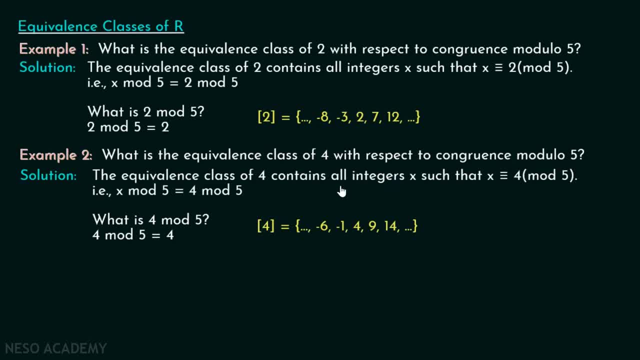 of four. with respect to congruence modulo five. The equivalence class of four contains all integers x, such that x congruent to four mod five, which means that x mod five must be equal to four mod five. What is four mod five? Four mod five is four Right. 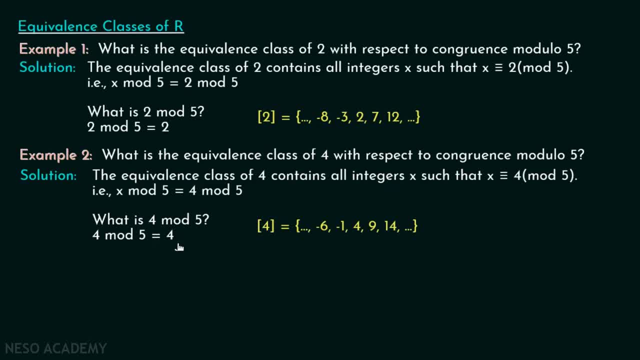 So including all those integers which will leave the same remainder four. we know that four must be included in this equivalence class. Apart from this, nine must be included, fourteen must be included, and so on. We can also include minus one and minus six. 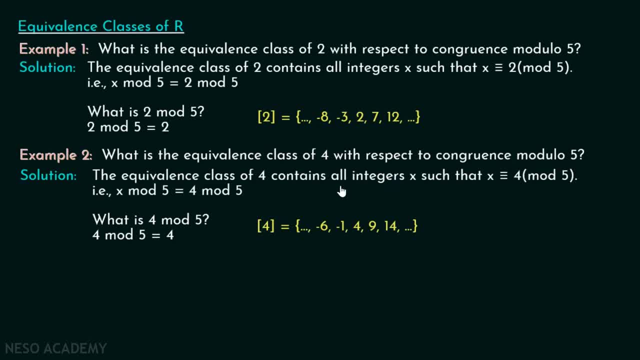 of four. with respect to congruence modulo five. The equivalence class of four contains all integers x, such that x congruent to four mod five, which means that x mod five must be equal to four mod five. What is four mod five? Four mod five is four Right. 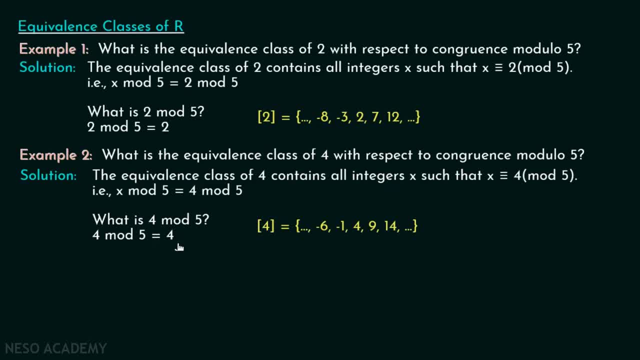 So including all those integers which will leave the same remainder four. We know that four must be included in this equivalence class. Apart from this, nine must be included, fourteen must be included, and so on. We can also include minus one and minus six. 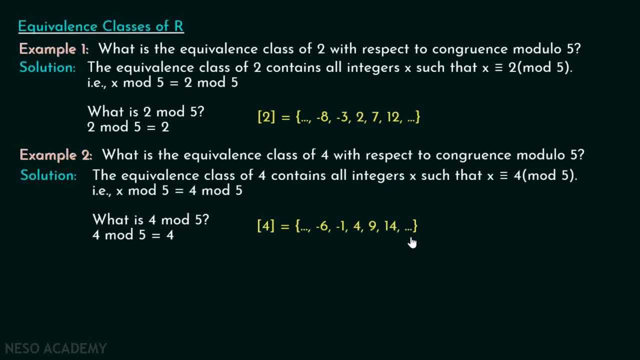 in this equivalence class, Right. This is again an infinite list. So equivalence class of four must consist of these elements and more elements which are represented by these dot dot dot, Right? So this is the equivalence class of element four. Two must be included in this equivalence class. 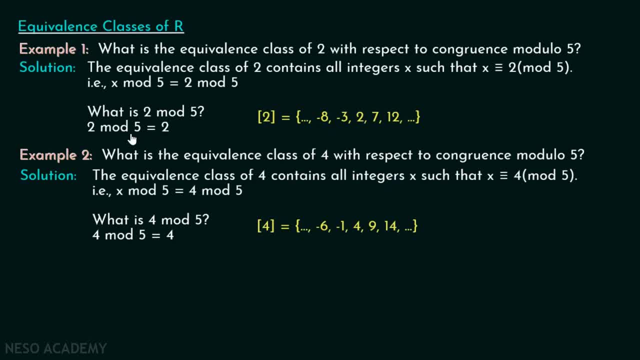 because two is the remainder when we divide two by five. Right Apart from this, seven must be included, twelve must be included, minus three and minus eight must be included, and so on. Right Here, seven is included, which is nothing but two plus five. 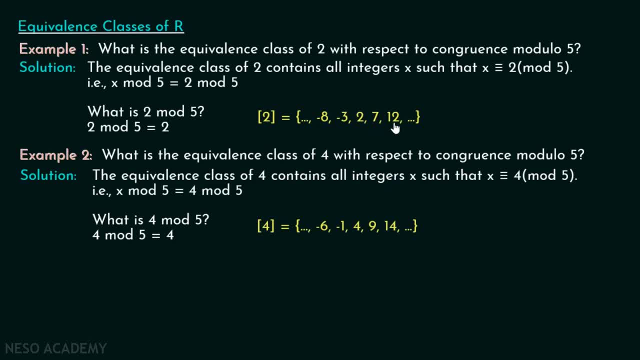 Right Twelve is included, which is nothing but seven plus five. It seems like we are adding this five to each element over here. Right Apart from this, we are subtracting five from this two in order to get minus three. We are also subtracting. 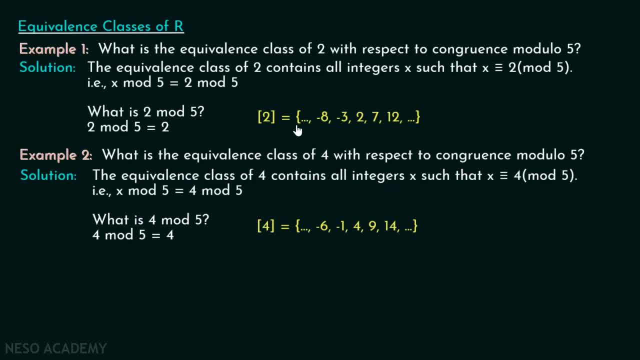 five from this minus three to get minus eight, and so on. In similar way, here also we are adding five to this four in order to get nine. We are also adding five in this nine in order to get fourteen, because here also we have five. 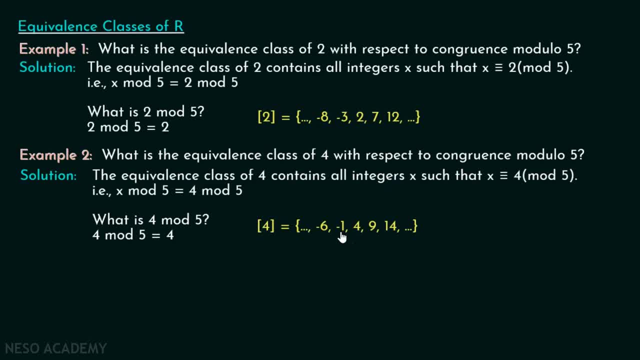 Also, we are subtracting five from four in order to get minus one, and we are subtracting five from minus one in order to get minus six. We can generalize these examples, in other words, Right Generalizing the examples, The equivalence classes of congruence, modulo m. 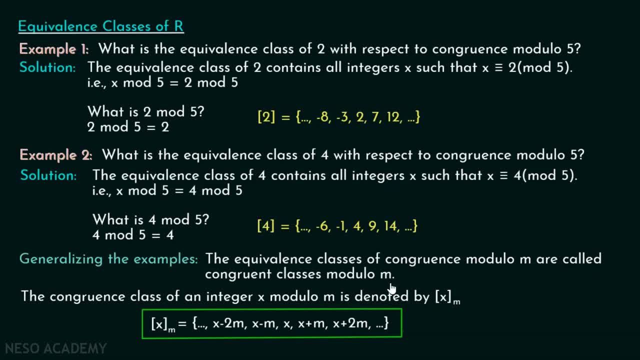 are called congruent classes modulo m. Let me tell you the equivalence classes of congruence modulo m are called congruent classes modulo m. The congruence class of an integer x modulo m is denoted by x in the square brackets: m. 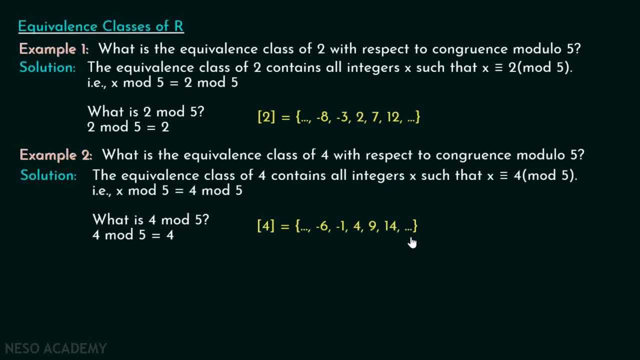 in this equivalence class, Right. This is again an infinite list. So equivalence class of four must consist of these elements and more elements which are represented by these dot dot dot, Right? So this is the equivalence class of element four. Two must be included in this equivalence class. 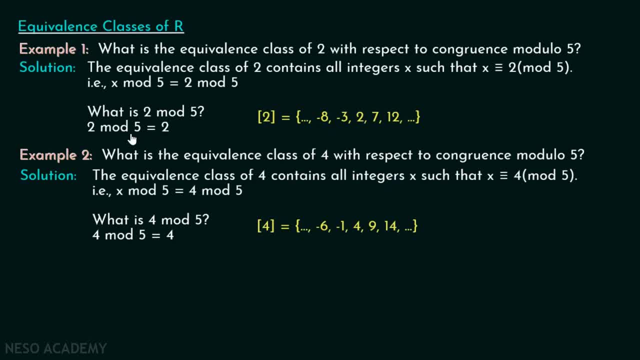 because two is the remainder when we divide two by five. Right Apart from this, seven must be included, twelve must be included, minus three and minus eight must be included, and so on. Right Here, seven is included, which is nothing but two plus five. 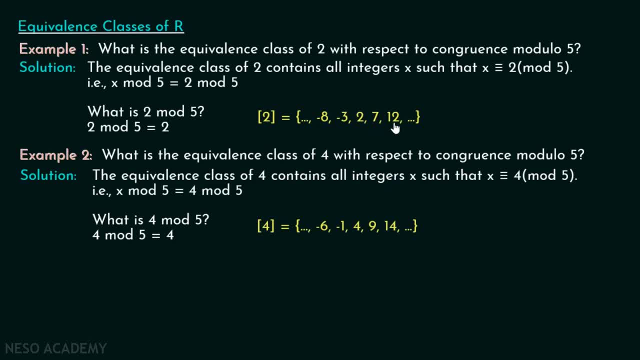 Right Twelve is included, which is nothing but seven plus five. It seems like we are adding this five to each element over here. Right Apart from this, we are subtracting five from this two in order to get minus three. We are also subtracting. 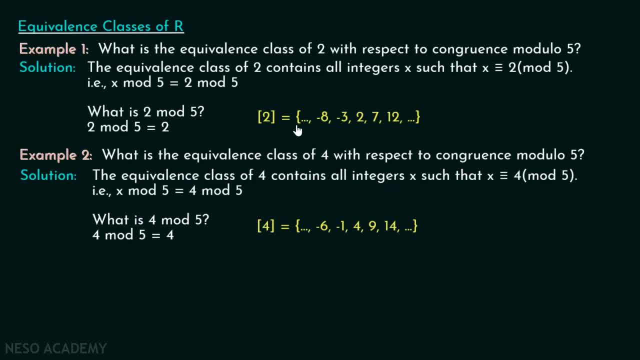 five from this minus three to get minus eight, and so on. In similar way, here also we are adding five to this four in order to get nine. We are also adding five in this nine in order to get fourteen, because here also we have five. 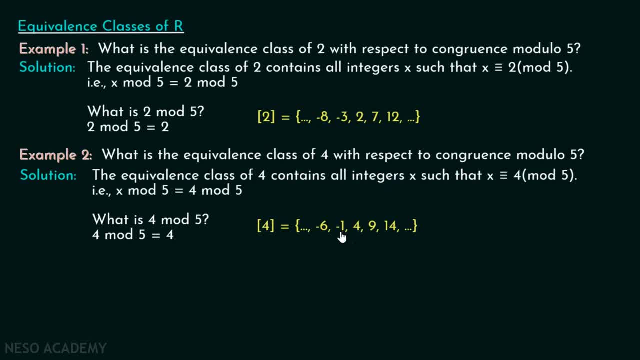 Also, we are subtracting five from four in order to get minus one, and we are subtracting five from minus one in order to get minus six. We can generalize these examples, In other words, right Generalizing the examples, The equivalence classes of congruence. 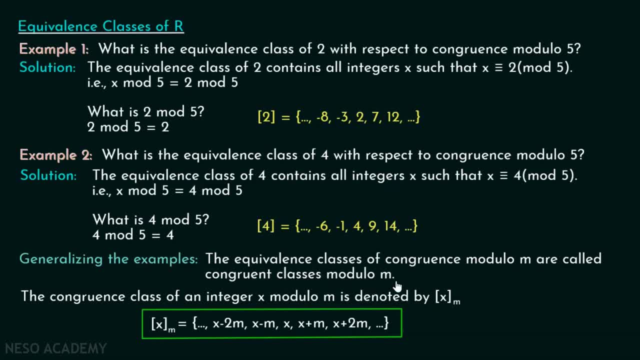 modulo m are called congruent classes modulo m. Let me tell you the equivalence classes of congruence modulo m are called congruent classes modulo m. The congruence class of an integer, x modulo m, is denoted by x in the square brackets, m. Okay, x, m is nothing but. 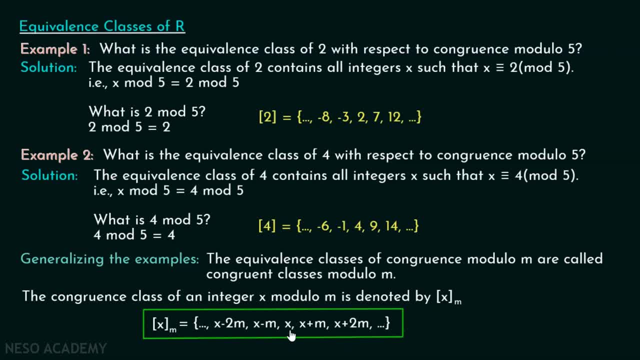 the set of all these elements where x must be included, This x must be included. Then we have x plus m, x plus 2m, and here we have x minus m, x minus 2m and so on. Right, This is x m. Fine, We have found this pattern from these examples, and this is applicable to all. 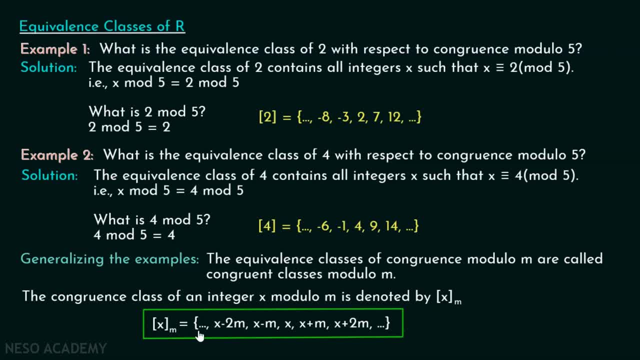 Okay, x, m is nothing but the set of all these elements where x must be included. This x must be included. Then we have x plus m, x plus two m, and here we have x minus m, x minus two m, and so on. Right, This is x. 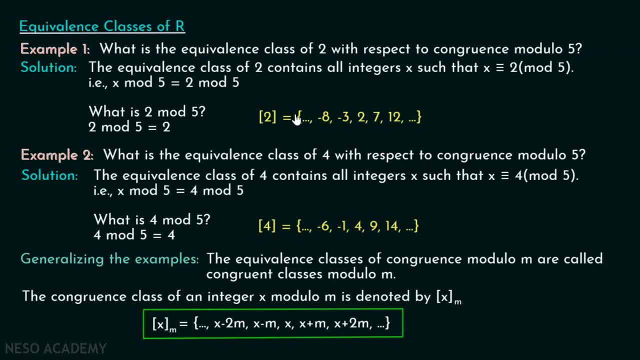 m. Fine, We have found this pattern from these examples, and this is applicable to all these type of examples. Right Now, let's see one problem related to this: congruence modulo m. What is the congruence class four m when m is? 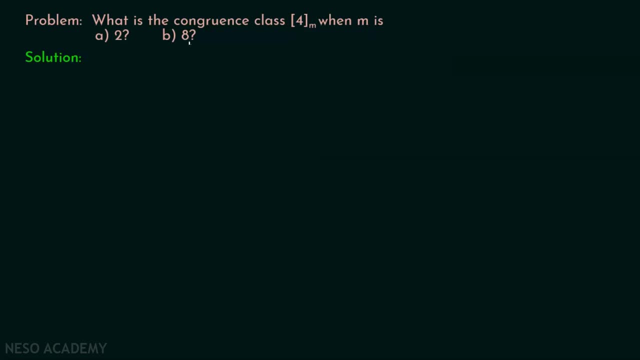 two, eight. Okay, Let's first take m as two. This means we are interested in finding four, two. This is nothing but set of all integers x, such that x is congruent to four mod two. We have seen the definition Right. This is nothing but set. 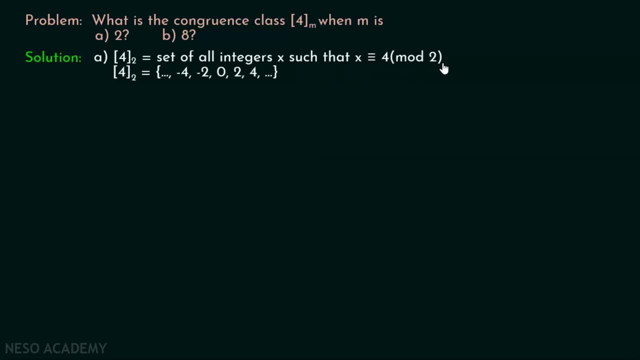 of all integers x, such that x is congruent to four mod two. We are interested in finding all those integers which will leave the same remainder as of four mod two. What is four mod two? Four mod two is nothing but zero. First of all, 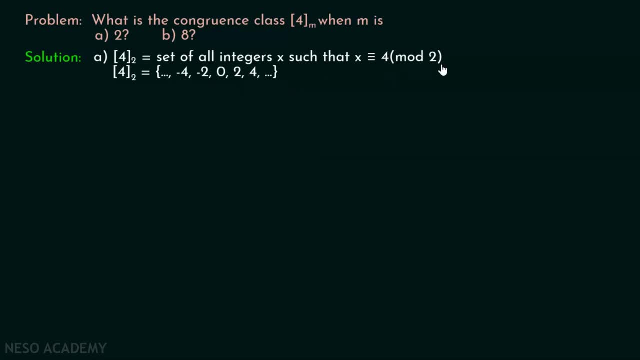 four must be included in this set Right, Because four mod two is equal to four mod two. Four must be included. Two must be included. Zero must be included. Minus two minus four. all these elements are included. Apart from this, we can also: 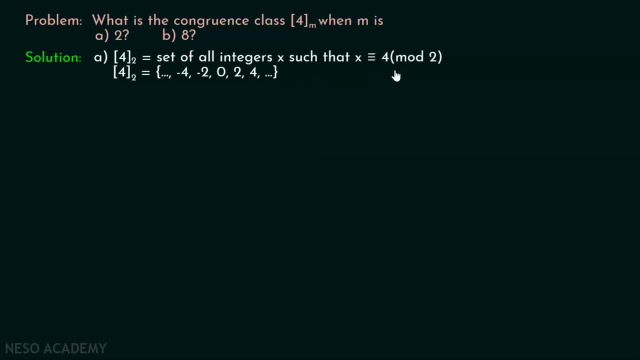 include six, because six mod two is also zero, Right, And we can continue like this. So this is the set which consists of all these elements, which leave the same remainder as of four mod two. Now, what about four eight? This means set of all integers. 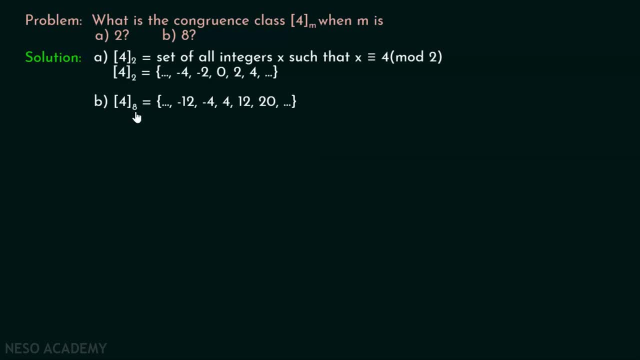 x, such that x is congruent to four mod eight. What is four mod eight? Four mod eight is nothing but four. Right Four must be included in this. set Apart from this, twelve, twenty and so on must be included. Then minus four, minus. 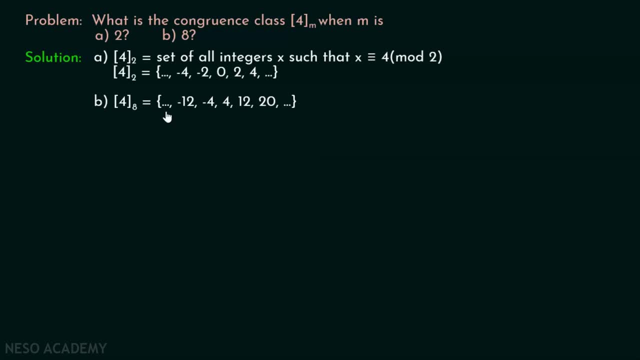 twelve and so on must be included, Right? So this is the equivalence class of four- eight. Now here is one homework problem for you. What is congruence class n- five when n is three, six and minus three? You can always post your answers in the comment section.